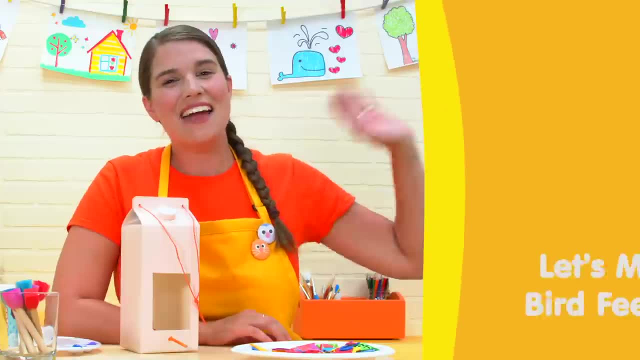 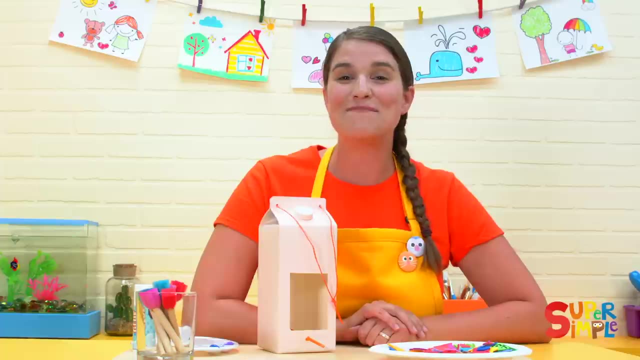 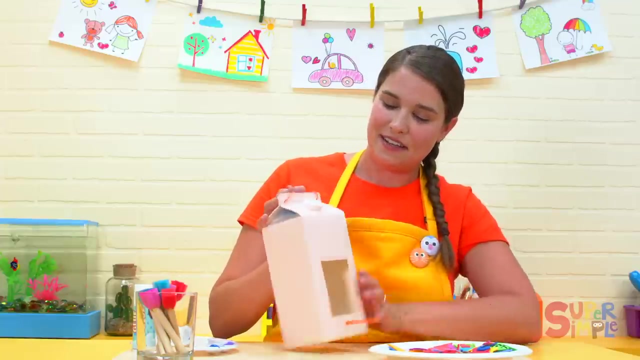 Hi everyone. I wanted to do something nice for the animals in my backyard, so I decided to try and make a bird feeder. I made one- this one- out of some recycled materials. I used an old juice carton and these things- sometimes they're juice, sometimes they're. 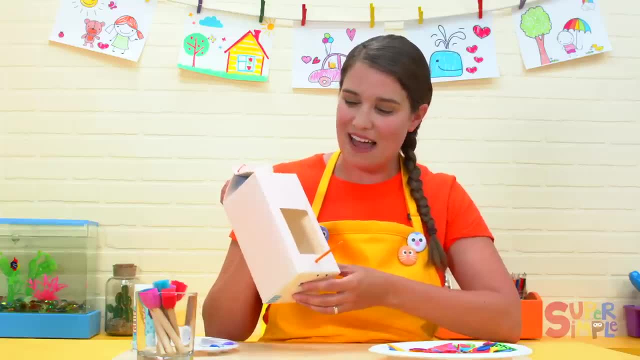 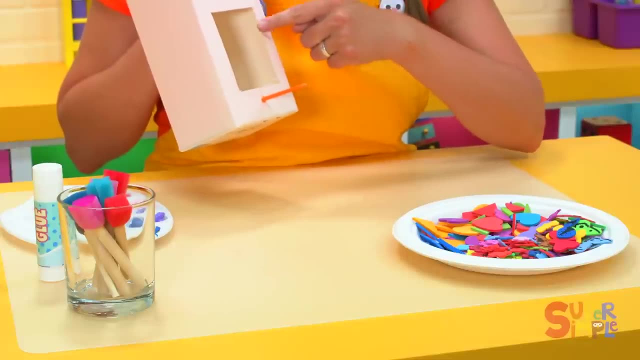 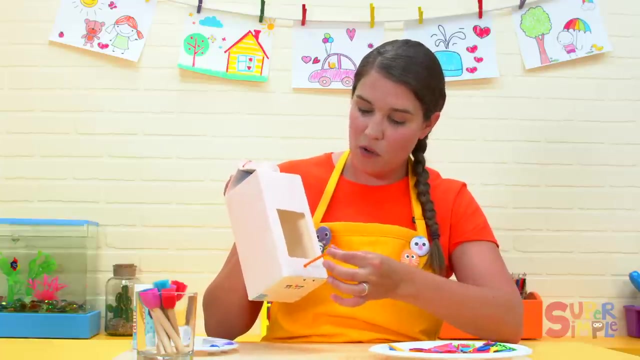 milk and I cleaned it all out- so it was nice and clean inside- and then very carefully cut a rectangle and that'll be the door to my birdhouse. Then I very carefully drilled and cut a hole here on either side, one hole for a wood stick to go through. It goes all. 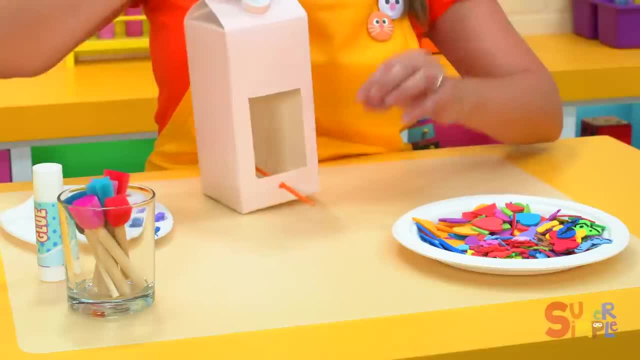 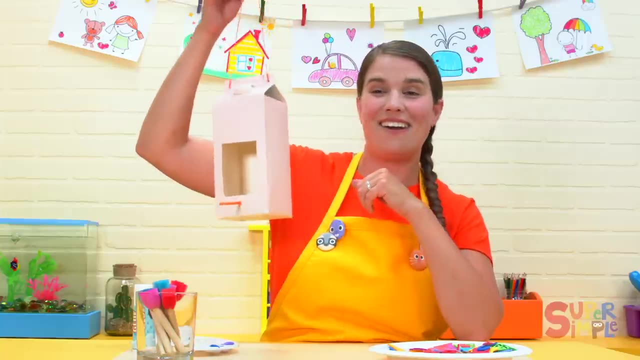 the way through to the other side and that's going to be the perch for the birds to sit and eat at the bird feeder. And then I put some string through the holes up here so it can hang on the tree, so it's at a nice place for the birds to get it. 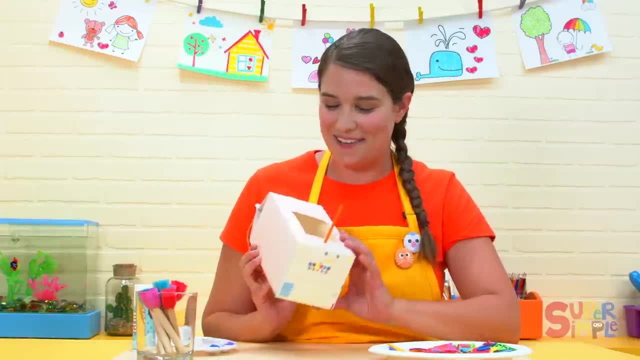 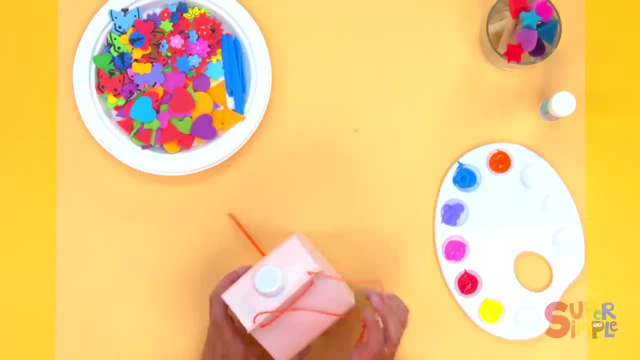 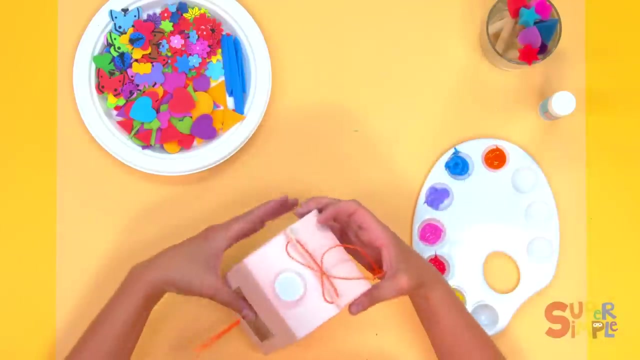 And all I have to do now is decorate it. I painted it before, so now it's nice and ready for some decorations. So I have some different stickers here and some different colors of paint, with some sponge stamps that I can use to decorate it. Let's give it a try. How about? 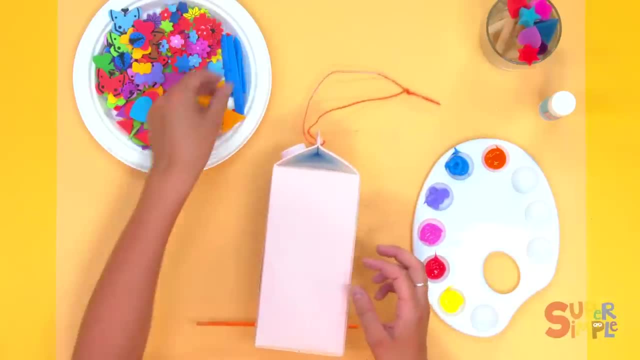 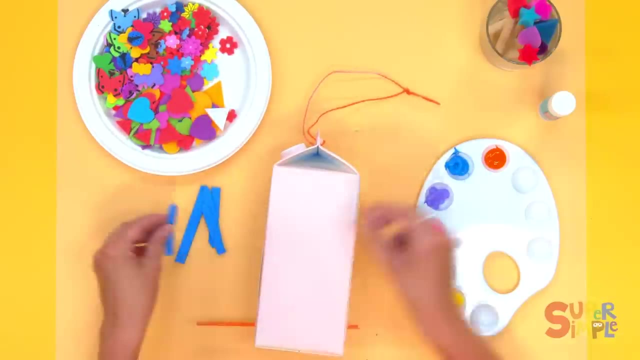 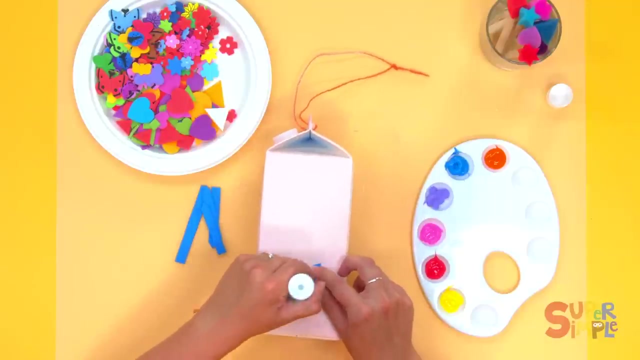 we start with. hmm, I cut out some of these pieces of foam to make a little fence along the bottom of the bird feeder. I thought that might be a good idea, A cute thing, so that birds can have their own little fence on their own little house. 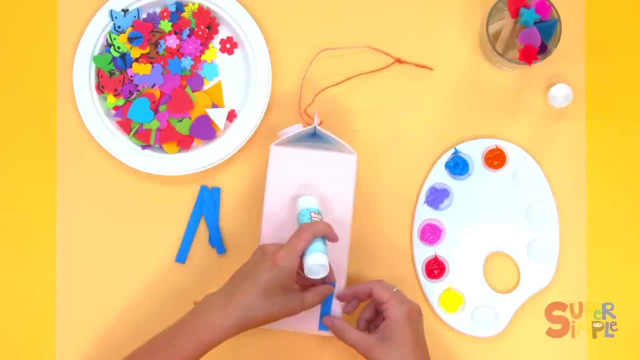 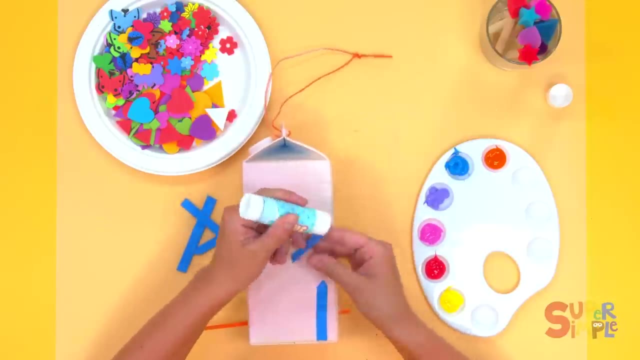 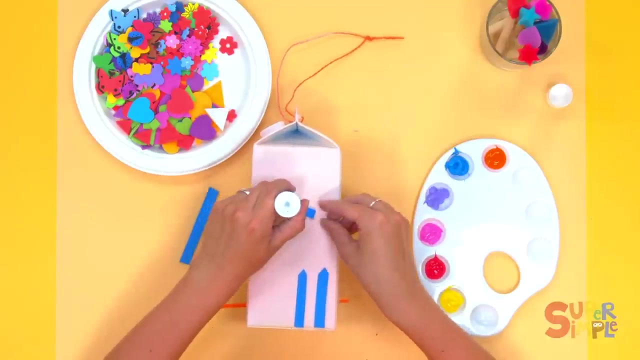 I'll use some glue to attach it to the bottom. here You can decorate your bird feeder any way you like. There's lots of different ways to decorate it. You could color it, put on stickers, use some paint or glue on some pieces like I am. How about one more? 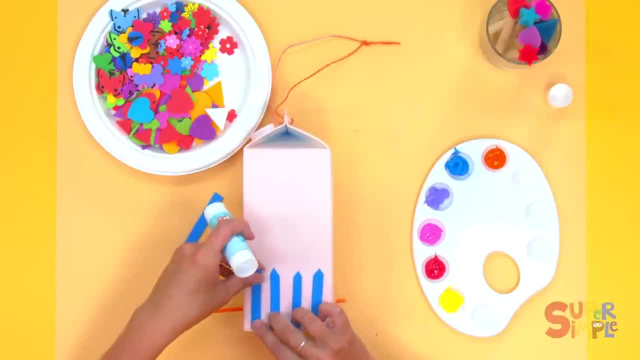 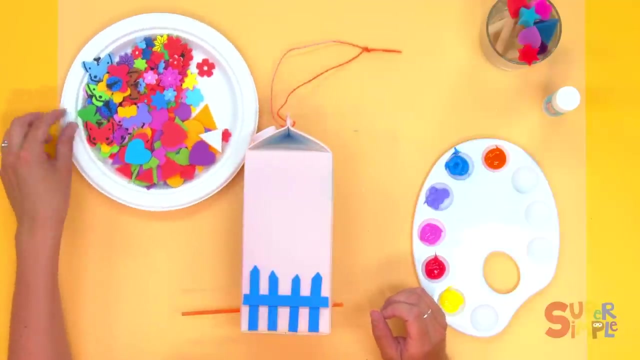 Here we go, Very nice, And then one piece to go across this way to complete our fence. Excellent, Ta-da, There's our beautiful fence. Okay, let's see what else we can add. How about? oh, I have some butterfly stickers. We can have some butterflies flying around. 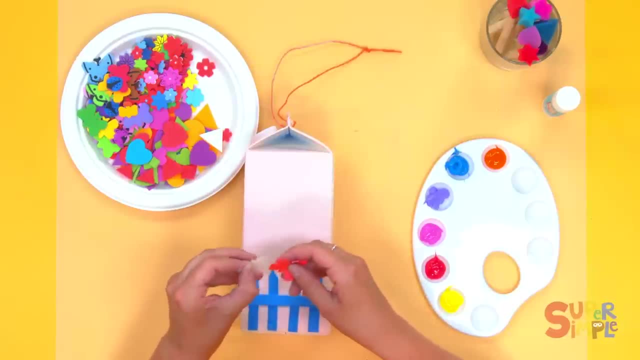 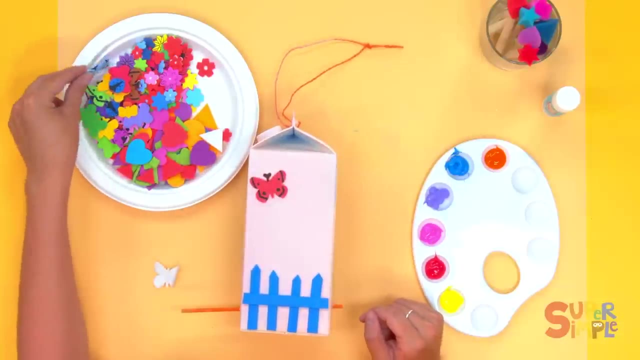 Okay, Let's see what else we can add. How about? oh, I have some butterfly stickers. We can have some butterflies flying around The bird house. Okay, we'll put one butterfly here. Here we go. How about a blue butterfly? 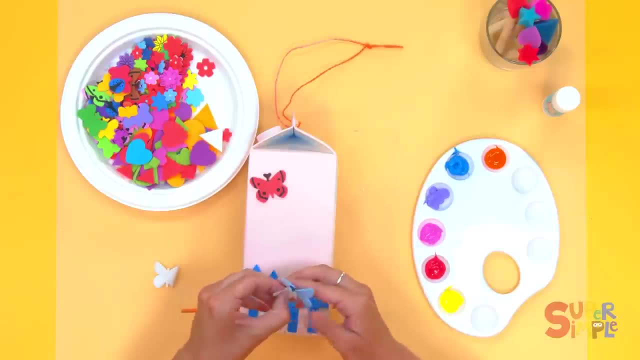 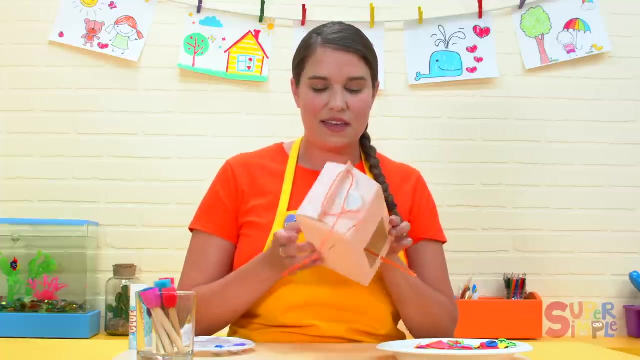 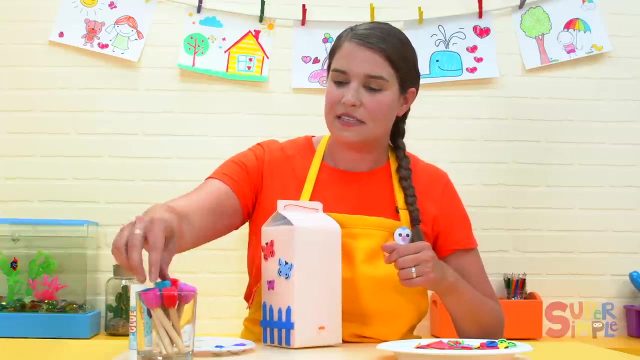 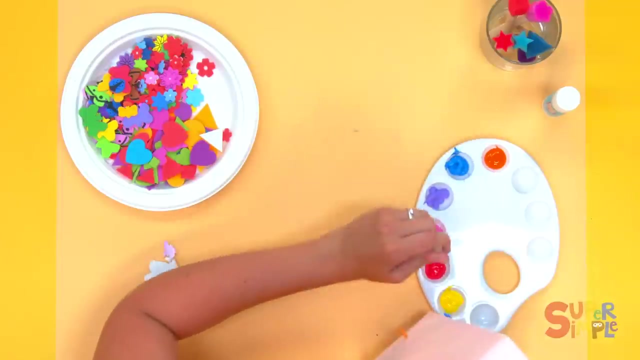 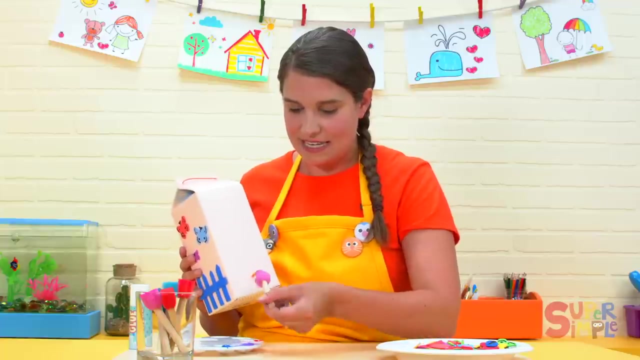 over here, So nice. And how about a little purple butterfly? Put it down here and they'll all be flying together. Here we go. That's beautiful. Okay, how about we add some stamps to the back of our bird feeder? I'll use some of these sponge stamps. I got some different shapes here. I can do a heart, We'll do some different colors, We'll do how about some red hearts? Dip it in the paint And it's just like a stamp. Here it comes. 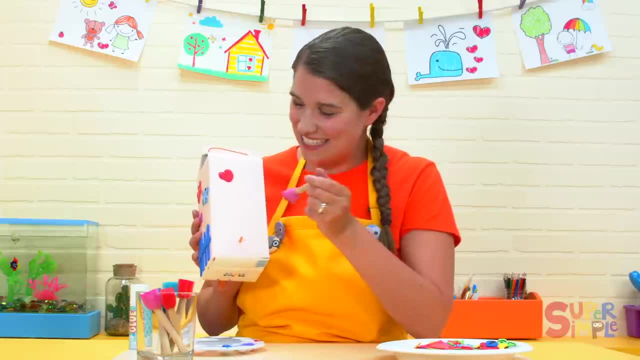 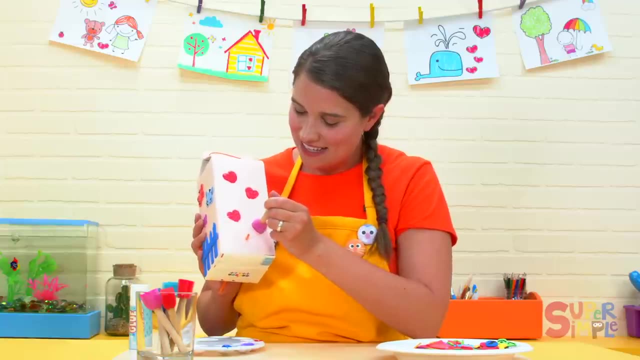 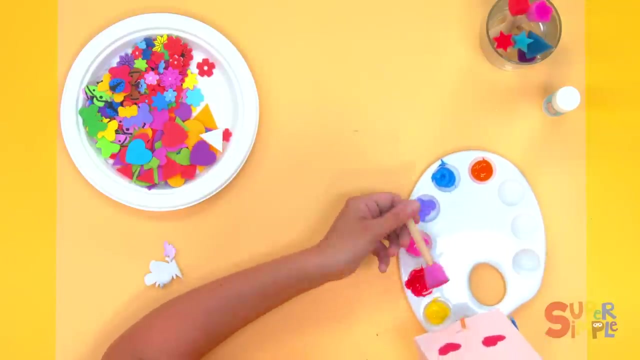 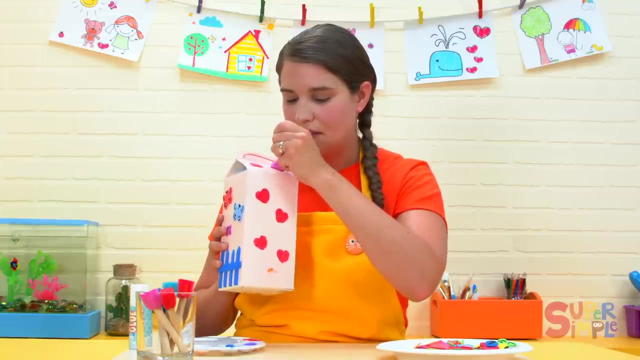 I can do a red heart. Here we go, There we go. Let's see how much we get on top of it. I think there's maybe three of them. Oh, so nice, Our red hearts, So pretty. How about up here we can make some red hearts too? 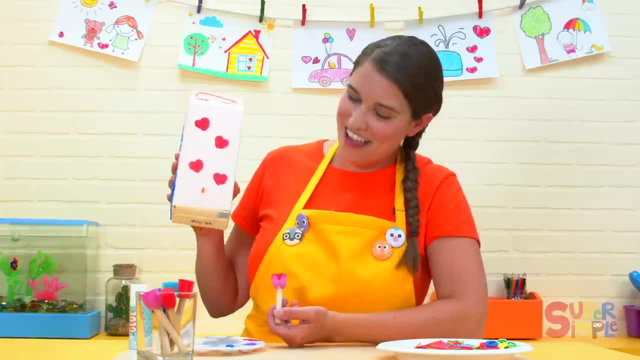 There we go, So nice. And red hearts for the birds, so they know they're loved. Oh, There we go. There we go, So nice. And red hearts for the birds, so they know they're loved. Let's add some more color, but on this side. 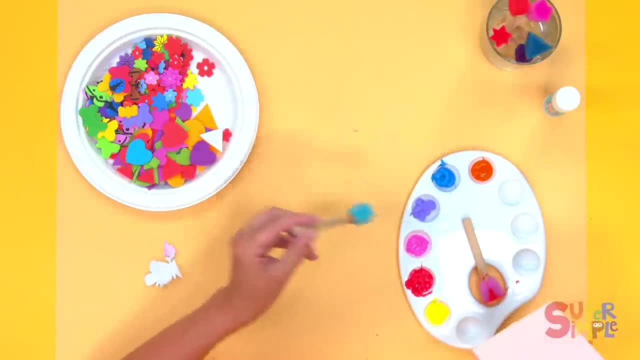 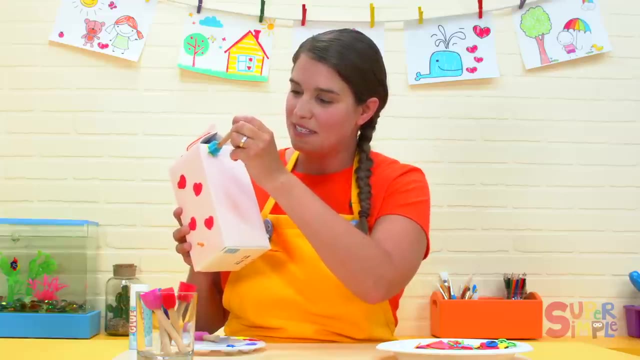 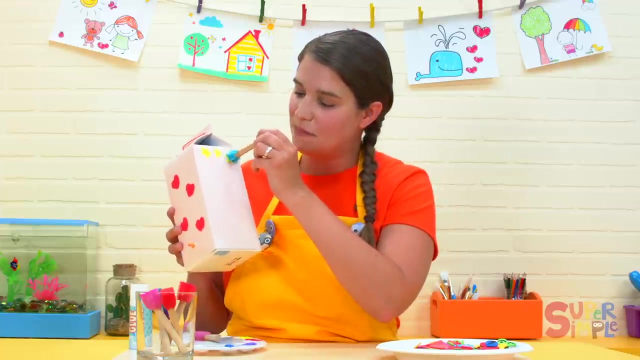 We'll maybe do some stars. What color should I use? Some yellow stars. We'll do some stars up here at the top, just like the night sky. I think the birds are gonna love this. It's nice to give the birds a place. 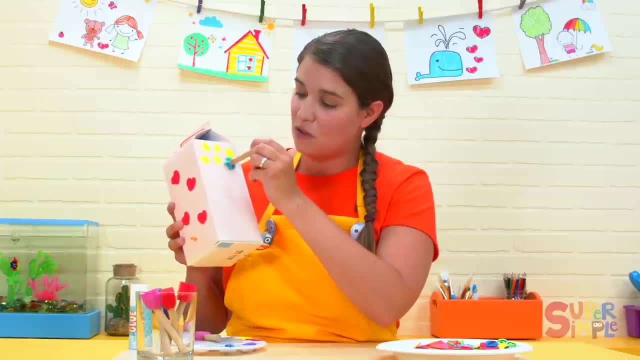 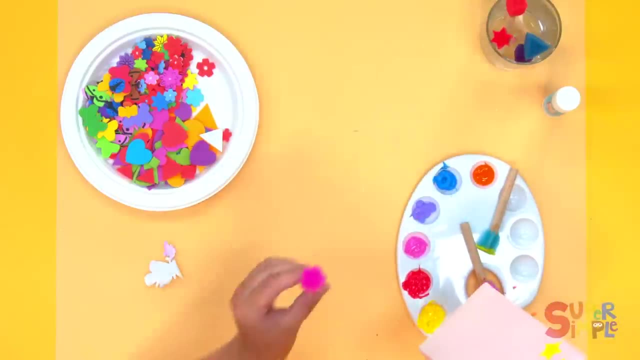 where they can safely eat, especially in the wintertime when it's cold And it's hard for them to find food. So it's nice to have a place where they can come and have some food. This one kind of looks like a flower. 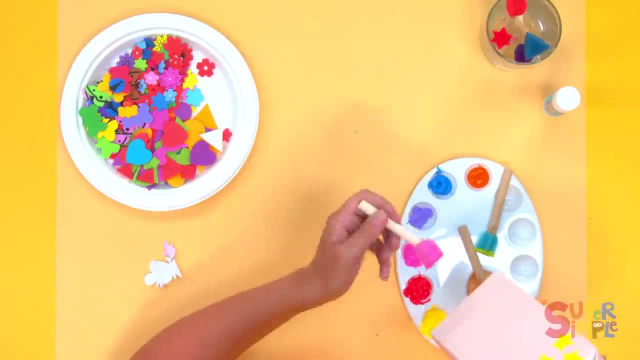 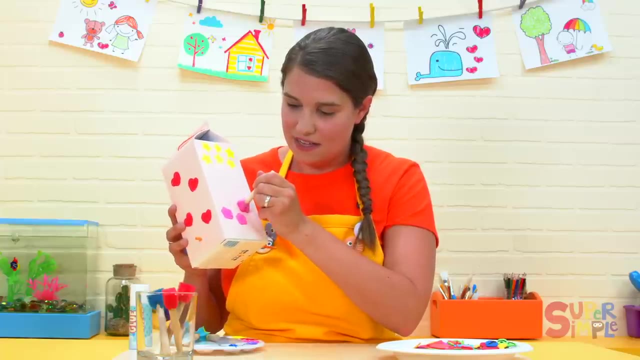 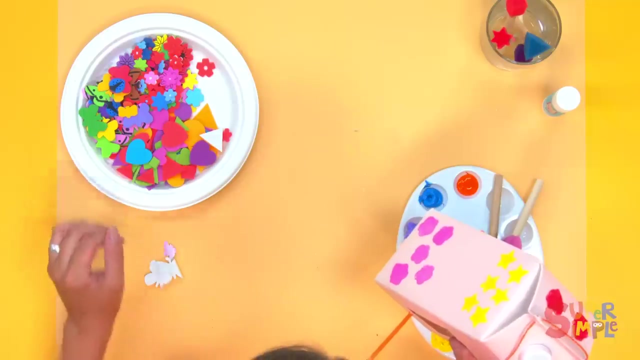 Let's do some pink flowers Down here. flowers grow from the ground. There we go. Those are beautiful. Get some more paint, So nice. Let's add something in the middle too. How about some shapes? I have some different stickers here of different shapes. 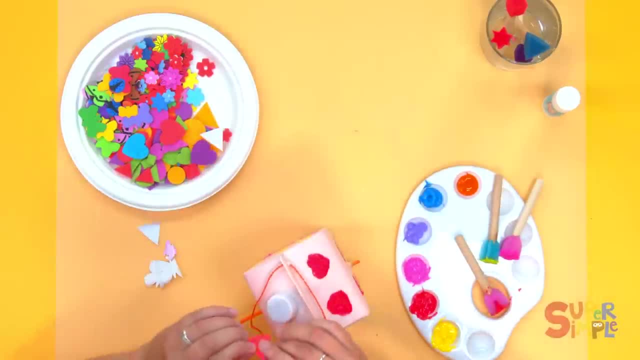 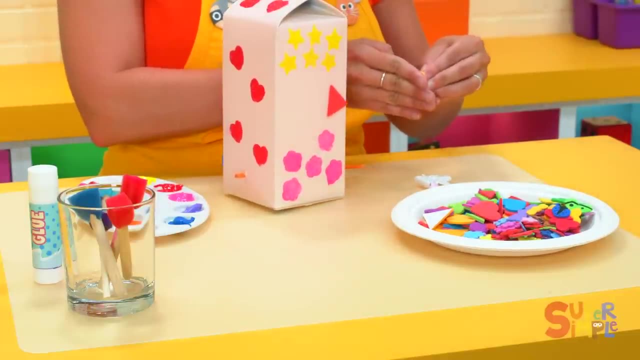 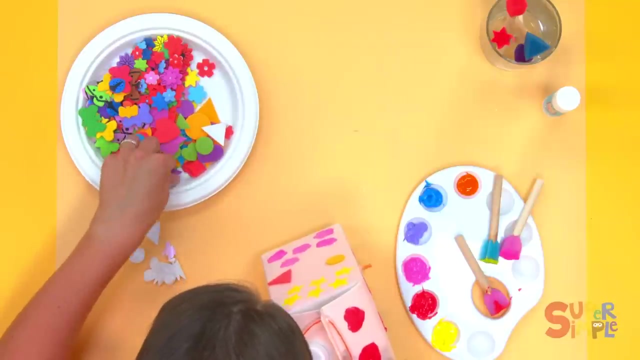 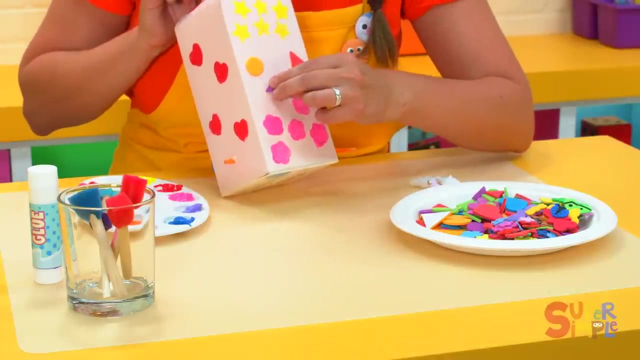 We can do a triangle, That one here in the middle. How about a circle? So a yellow circle, Ta-da. How about a purple triangle? Nice, I like all these colors. Let's add one more. How about a blue circle? 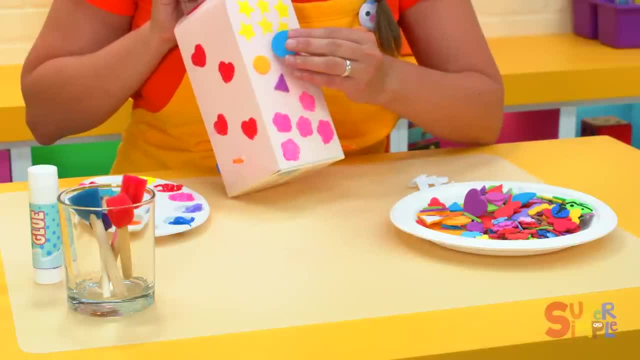 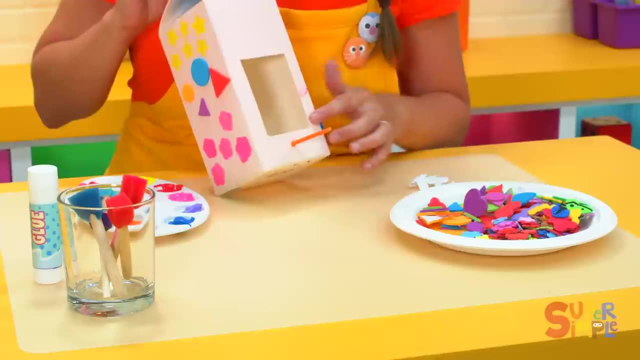 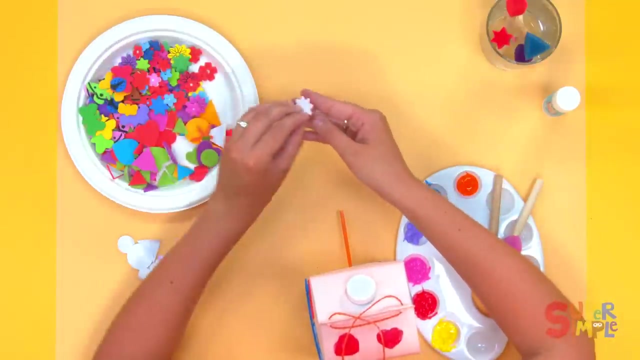 There we go. Look at all that So nice. Okay, let's decorate the front of our bird feeder now. This is the part that the birds are gonna come and eat at. How about we add some flowers? I have some pretty flower stickers here. 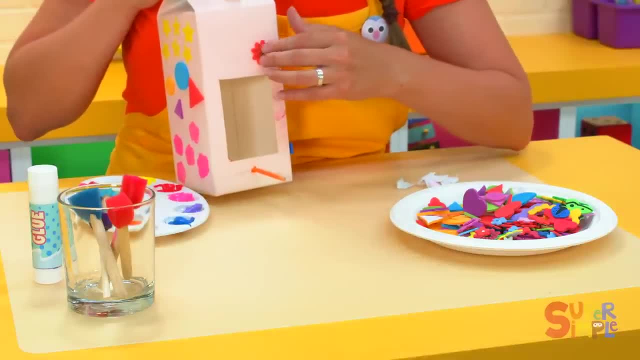 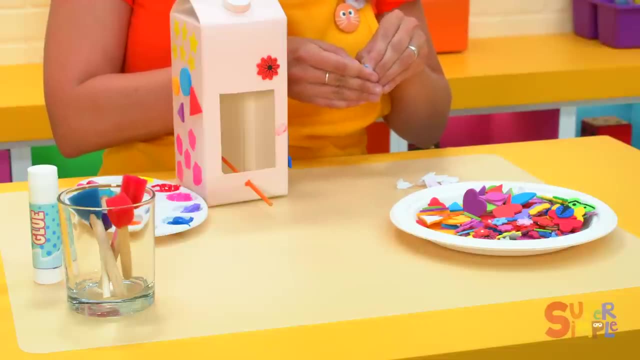 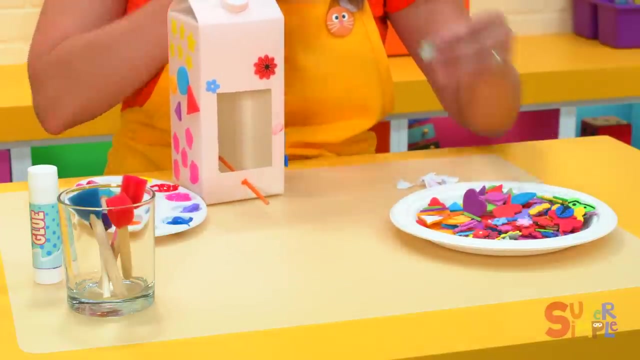 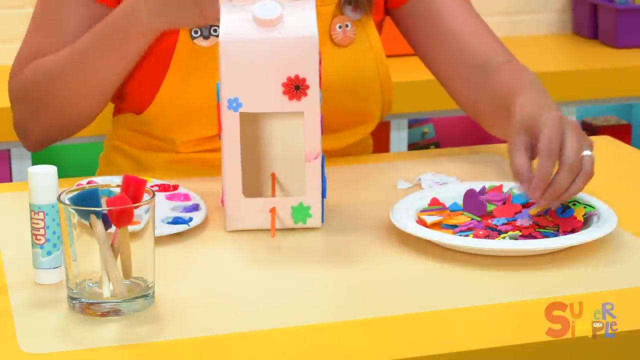 I'm gonna put some all around their door. Got a blue flower, So nice, And a green flower Down there, maybe. How about a yellow flower? I have a green flower in here. I'm gonna put a little bit of pink right up here. 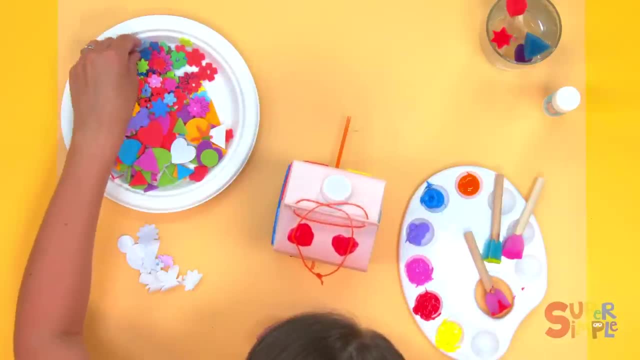 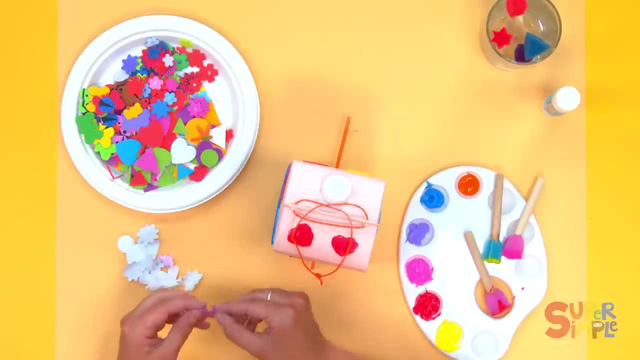 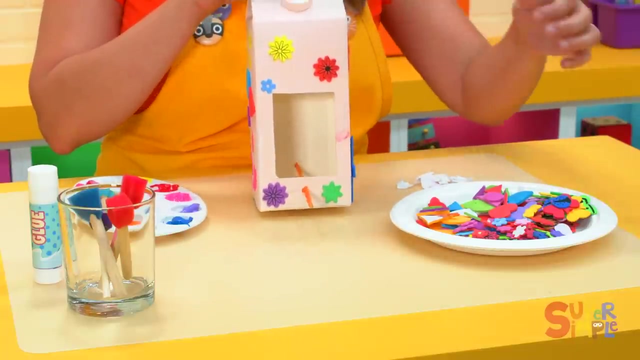 This is looking great. I think a couple more flowers will do the trick. How about this purple flower? Nice, big purple flower down here? Yeah, What else? How about one more up here? Okay, let's find a nice color, Nice big, bright color. 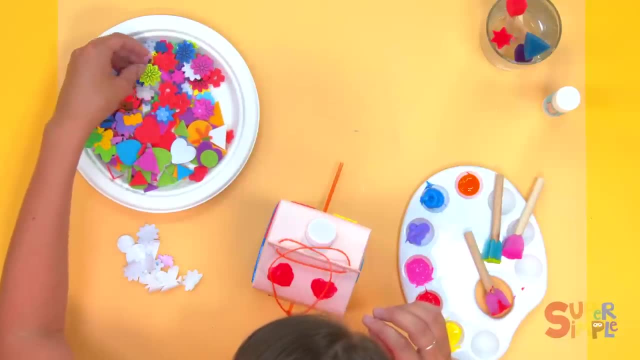 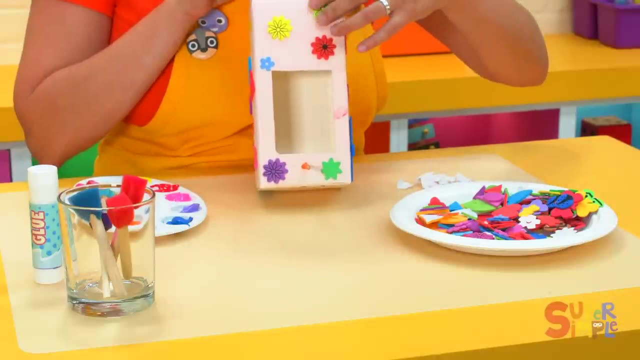 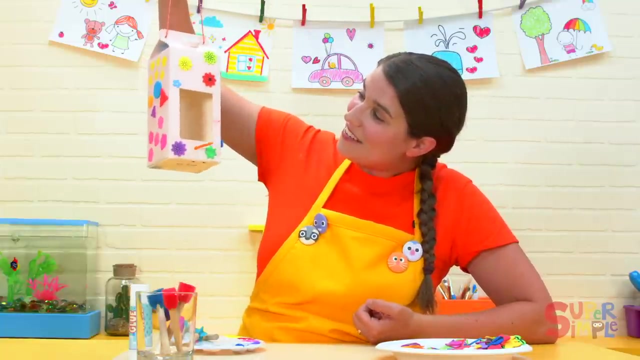 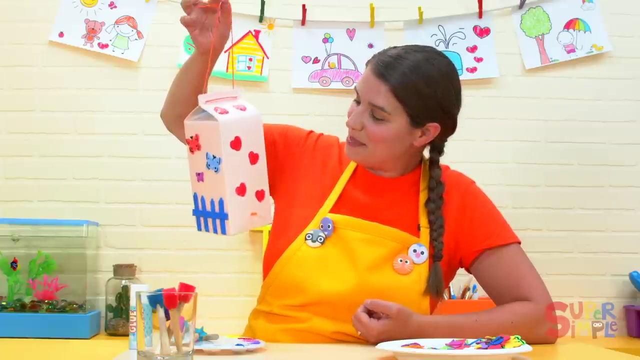 How about I like this one? it's kind of like a yellowy green. let's try this right up here. so nice. let's take a look at our bird feeder. got some flowers on this side our fence and the butterflies, our heart stamps, our stars and flowers and shapes. 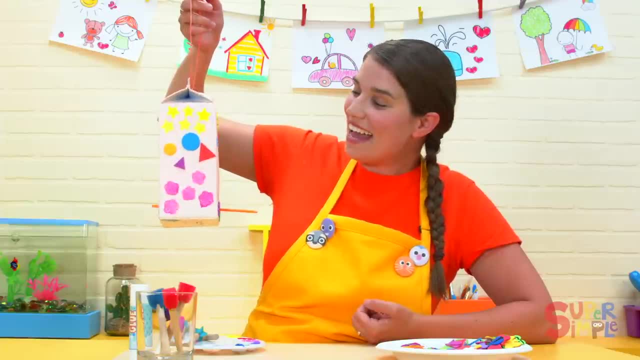 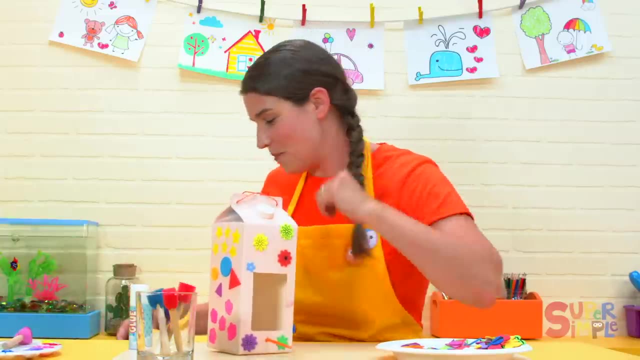 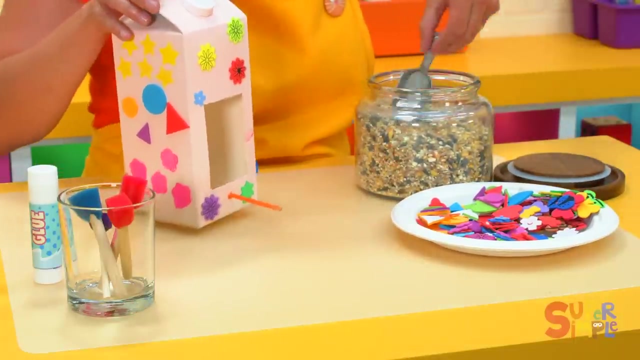 it's so nice, it's almost ready to go outside for our birds. but first we have to make sure the birds have something to eat. so let's add some. here we go. birds like to eat bird seed. it's got a little spoon here and i'll put it inside.